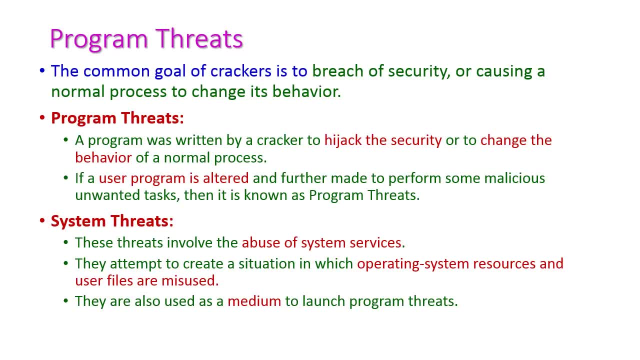 all those things one by one. Before that, let us discuss something about the program threads. The common goal of crackers or attacker is to break the security of system or causing a normal process to change its behavior. This is the common goal of cracker or attacker. Here there are two types of 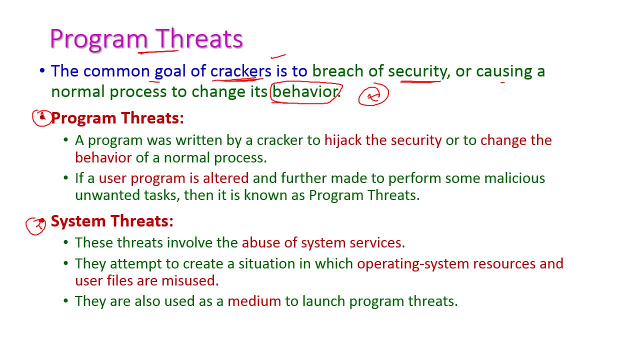 threads. First one is program thread and second one is system thread. Let us see program thread first. The program was written by cracker to hijack the security or to change the behavior of normal process. So the program that will hijack the security or change the normal behavior of the process is called as program. 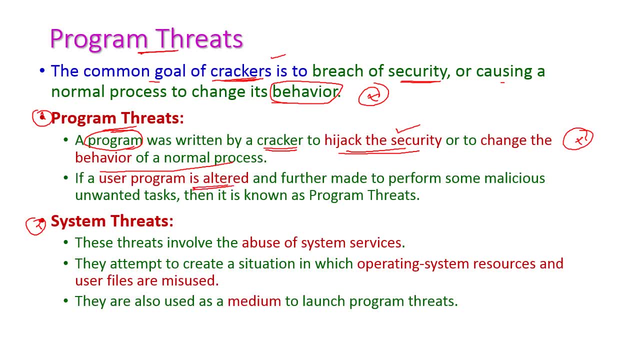 thread. If the program is altered, that is, if any of user program is altered and further made to perform some malicious, unwanted task, The normal program will be altered to do some unwanted task. this is known as program threat. right, okay. next one is system threat. here the 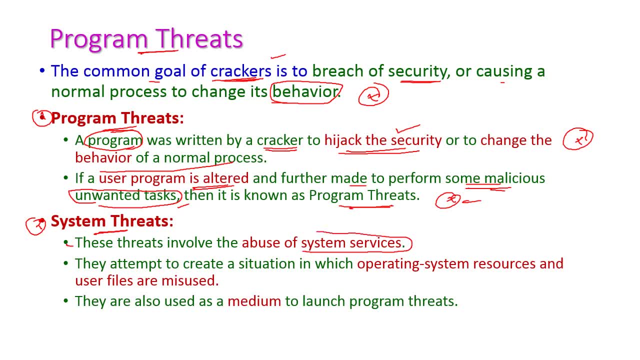 threats are involved. abuse of system services- right, okay, they attempt to create a situation in which the operating system resources and the user files are misused. okay, misusing their resources and user files are called a system threat. they also use a medium medium means, the communication medium to 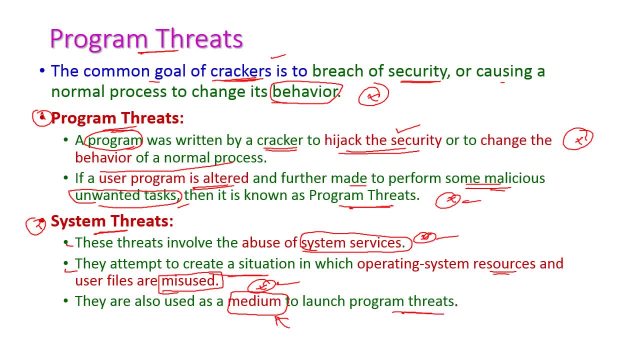 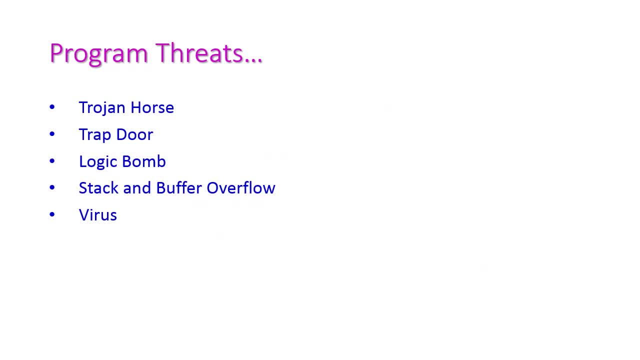 launch the program threats. okay, by using any of the medium like internet, they can launch the program threats in the computer system. some of the standard program threats are Trojan horse, trapdoor, logic bomb stack and buffer overflow and virus. let us see these things one by one. the first one is: 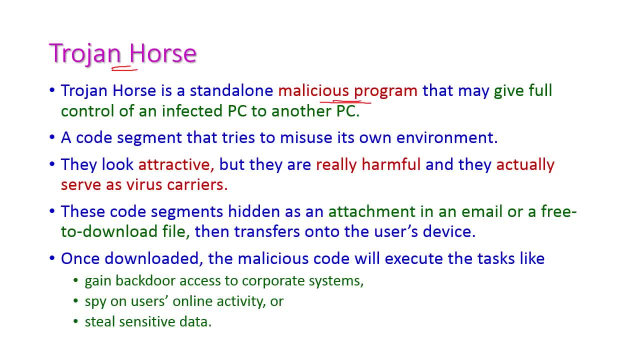 Trojan horse. it is a malicious program that may give full control of an infected PC to other PC. okay, here the Trojan horse is a code segment that tries to misuse its own environment. okay, see, this is our system. once the Trojan horse entered into our system, then the full control of this particular PC will be taken care of. the 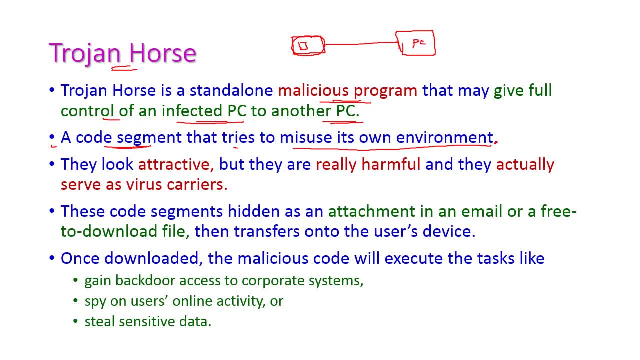 other PC. okay, from this PC we can control the affected PC. okay, and the malicious programs are actually looks very attractive, but they are very harmful and they actually serve a virus carriers. okay, and these code segments, that is, the Trojan horse, are hidden as attachments of emails. a free to download files and transfer to users devices. this 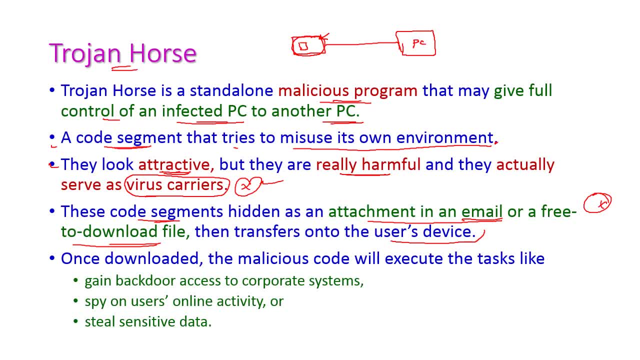 is how the Trojan horse files will be transferred to the user device. okay, once the file got downloaded, the malicious code will execute the task, like again, backdoor access to corporate system, spy on users online activity or steal the sensitive data. hence we have to careful while downloading the free attachments of email and free downloaded. files or any attractive advertisement from this 않는ный 598 00, forgive you know, and free downloaded files or any attractive advertisement from the developer related by anyone. you may have included おen and free downloaded files in the deviceешь surroundings. you have to be careful that this manage Del usage is actually. 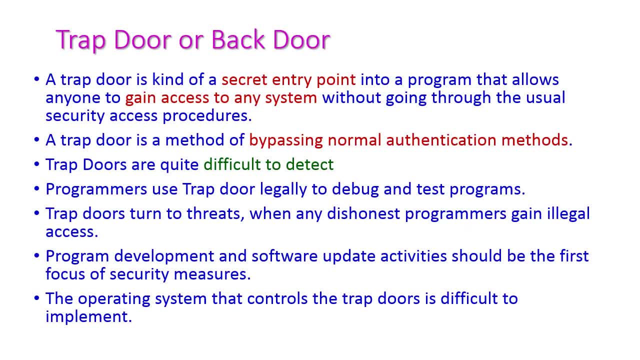 the internet. The second one is trapdoor or a backdoor. It is a kind of secret entry point into the program or the system which allows to gain the access to any system without going through the usual security procedures, That is, without any security procedures. the trapdoor- 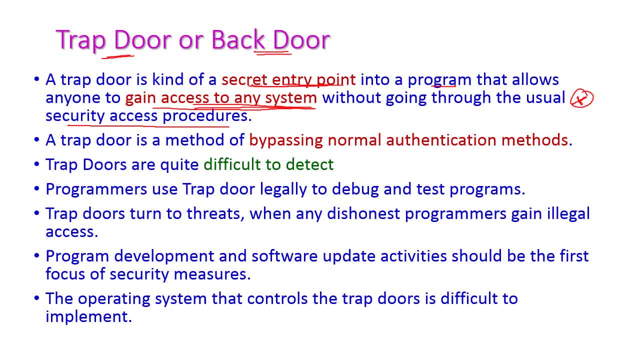 program can access all the system activities. It is a method for bypassing normal authentication methods and it is quite difficult to detect. So detecting trapdoor is very, very difficult. Normally programmers use trapdoor legally to debug and test the programs When it will. 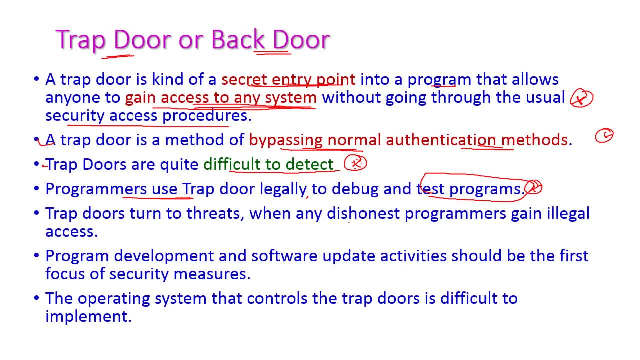 become illegal when the dishonest programmer gain illegal access. If it accesses illegally and threat all our programs, then it will become illegal, It will become a trapdoor. The program development and software update activities should be first focus, the security measures, But when come to operating system, the control, the trapdoor. 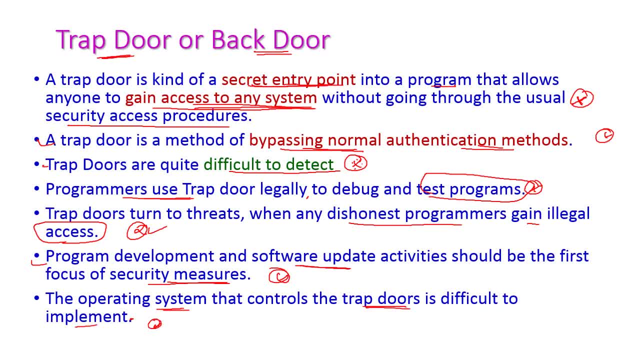 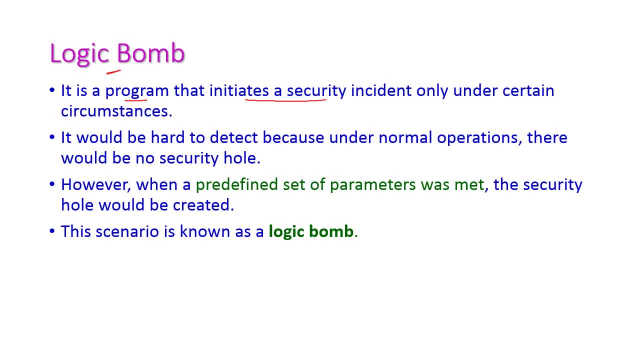 is very difficult to implement. The third one is logic pump, A program that initiates a security incident only under certain circumstance, And this will be very difficult to implement. This is very hard to detect because under normal operations there would no security hole. Ok, when a predefined set of parameters met, the security hole will be created. This 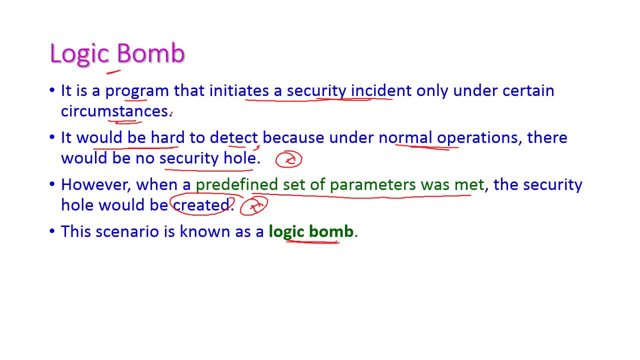 is called as logic pump. So under normal circumstance there is no security issues. But when a predefined set of parameters met, then the security hole will be created. This will be created. This is called as logic bop. The next one is stack and buffer overflow Here. 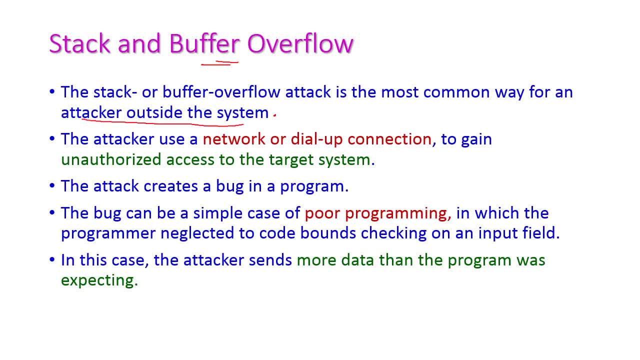 the attacker will stay outside the system and they will use network or dial-up connections to gain unauthorized access to the target system. Okay, here the attacker creates a bug program, that is, an error program that will be injected to the target system and the bug can be simple case of: 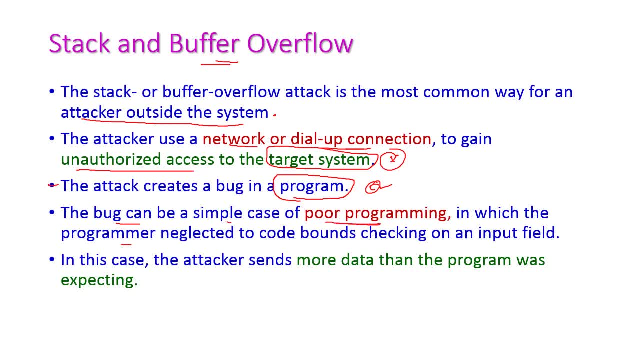 poor programming Okay, in which the programmer neglected to code bounce a check on the input field. They will check only the input field, not the program. So in this case the attacker sent more data than the program was expecting. Hence the stack will be overflowed or buffer will be. 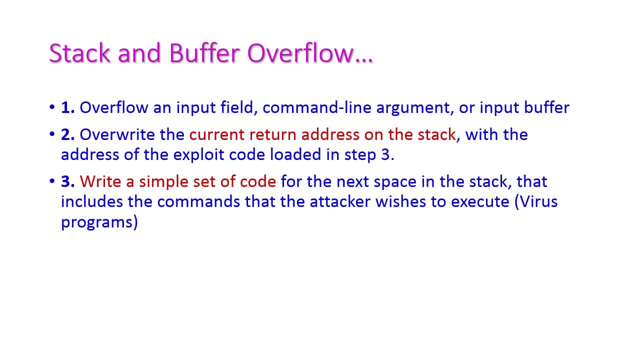 overflowed. For this, the attacker will follow three steps. The first step is overflow the input field, command line argument and buffer. that is, input buffer. Everything will be overflowed and overwrite the current return address of the stack. Okay, once the stack got overflowed, then the current return address will be changed with the. 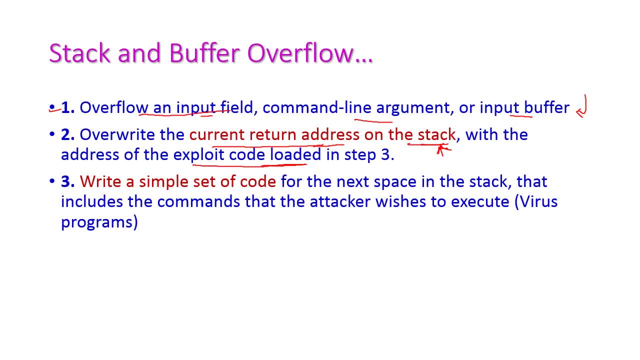 address of exploit code loaded in the step 3.. Okay, that means write a simple set of code for the next space in the stack. Okay, once the stack got overflowed, then, where the data will be stored. for that they are writing a simple code and the next data will be stored in some other program.